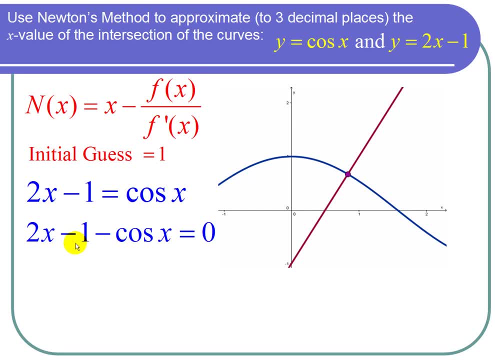 solve this. This definitely needs Newton's method. So I'm going to allow f of x to be the left-hand side of this equation: 2x minus 1 minus cosine of x. I need f prime of x because it's in Newton's. 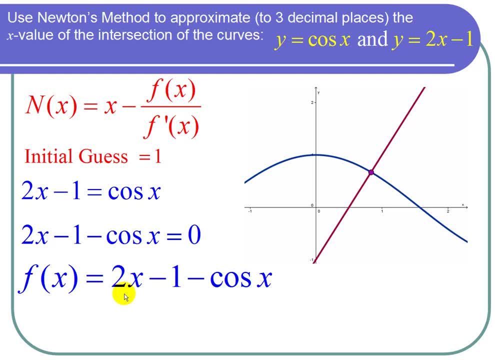 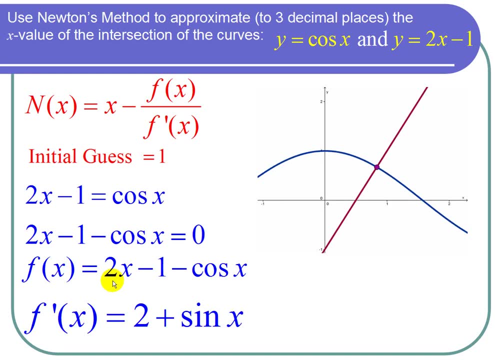 method formula. And f prime of x is the derivative Derivative, 2x is 2.. The derivative cosine is negative, the sine, So negative, negative, the sine is plus the sine And the 1 goes away. So at this point I can plug it into Newton's method formula. 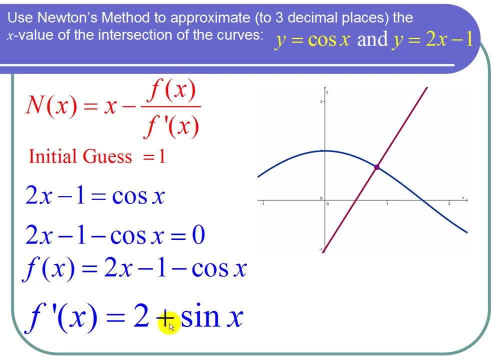 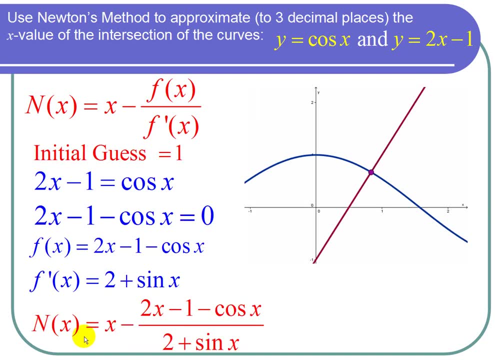 And I know that the next value of x is going to be x minus f of x. Here's f of x over f prime of x And here's f prime of x. So I'm ready for a table. I will have my guess number. 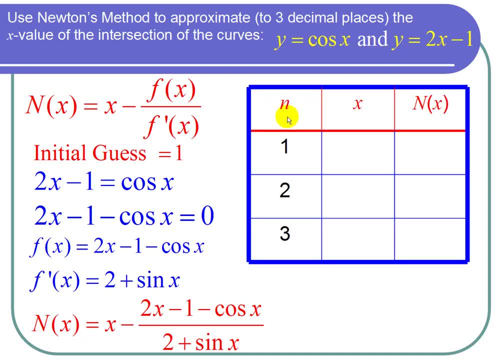 my x value that I'm plugging in and my Newton's method formula that gives me my next x value. So remember, my initial guess was 1, because that was pretty close to where they intersected. So that's my n equals 1.. x will be 1. And I used a calculator. 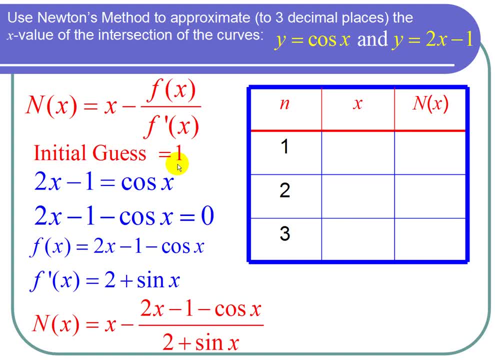 and I plugged in 1 into the n of x formula And I got 0.838.. I'm keeping three decimal places because that's what I'm asked to do. So then my next x value is 0.838.. So this is called a recursive function, where you take the value of x, you plug it in. 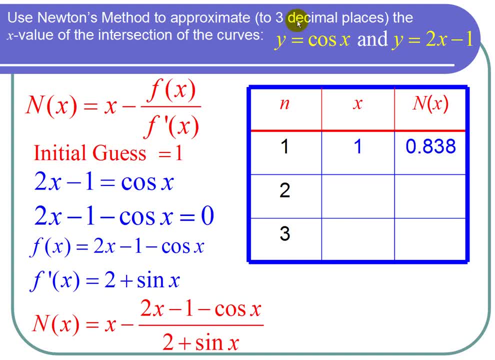 and you use what you get for the next value of x. And then you keep going. So now I'm going to plug in 0.838 into x in our Newton's method formula And I got 0.835.. And that will be my next x value. And then I need to plug in 0.835. 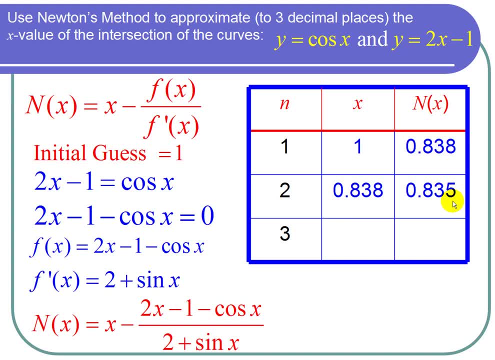 into my n of x function And again I got 0.835.. And that's wonderful, because when we repeat, plugging in 0.835 is going to get 0.835 forever. So that means up to three decimal places.